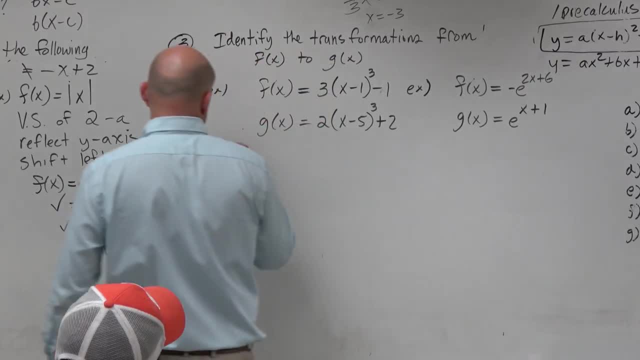 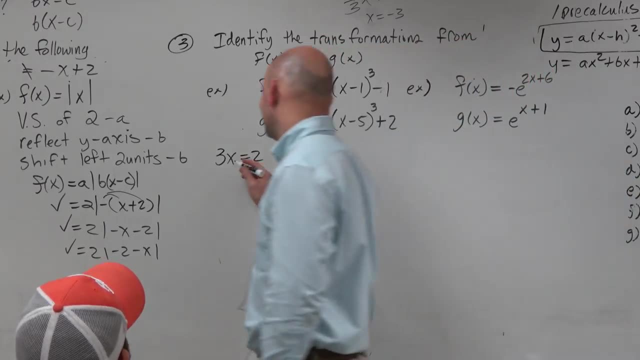 And some of you might say: oh, I don't know. Well, let's algebraically write it out Three times: what equals two, 2 thirds, 2 thirds. Right, That's the factor, And let's see if that makes sense. 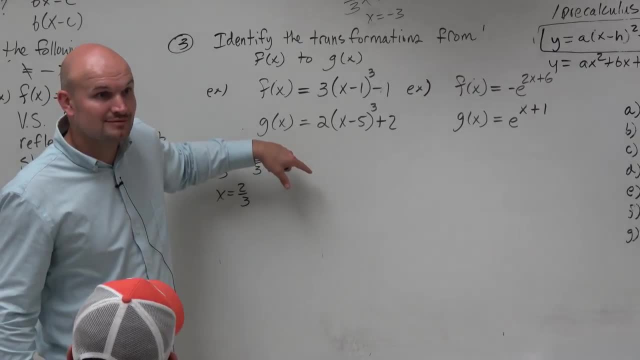 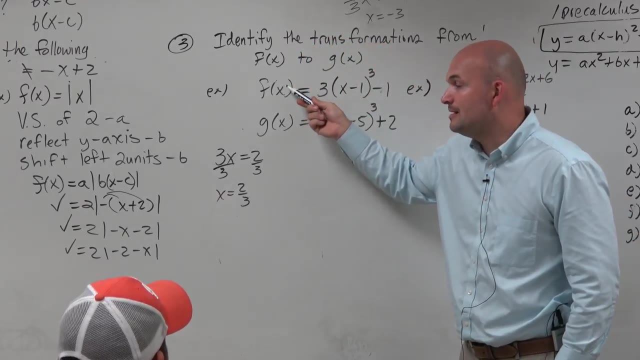 If I multiply three times 2 thirds, don't you get two? Two, Yes, You're going to have to multiply by three, Right? So if I have to multiply this function by 2 thirds, so that means I'm going to have to multiply on the outside. 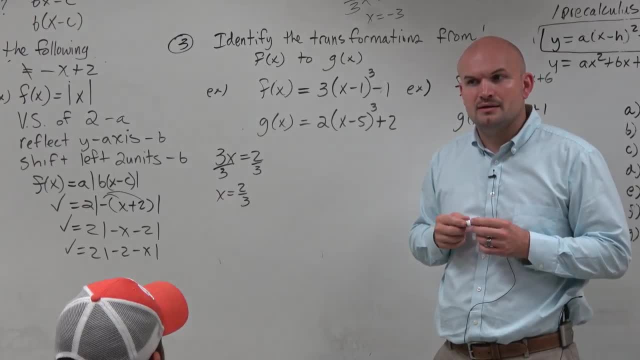 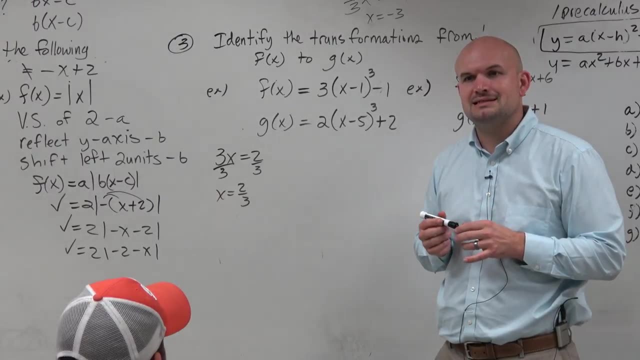 by 2 thirds. What would that be? First of all, it's going to be vertical right Because it's outside. But is that a stretch or a compression? It's a stretch, correct, It's a stretch, It's a compression. 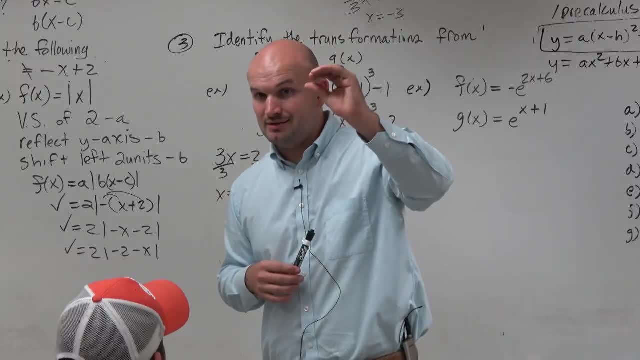 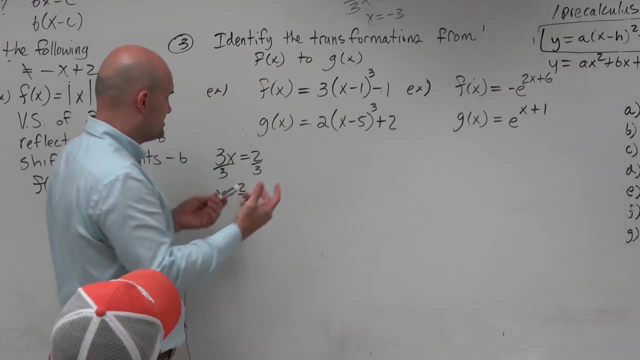 Well remember, the definition is: if it's larger than 1,. greater than 1, it's a stretch, If it's between 0 and 1, it's a compression. So 2 thirds is obviously less than 1.. 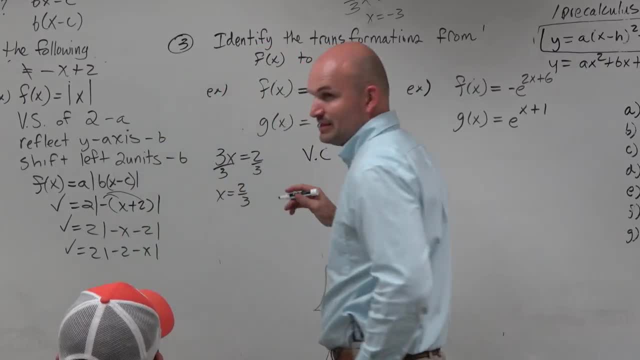 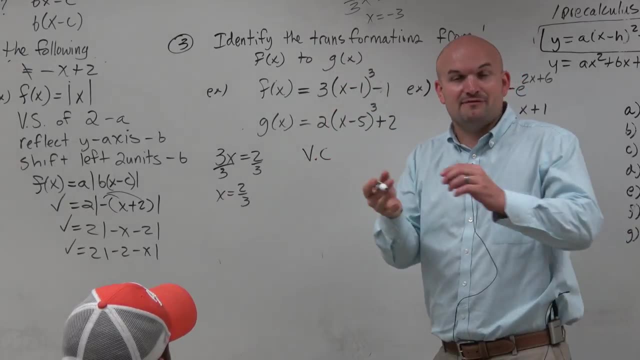 It is a vertical compression. One of the easy ways that we get people on this is: I could give you guys: what if I switch these around? What if I went from 2 to 3? Doesn't that make sense? If you go from 2 to 3, you'd have to multiply by 3 halves. 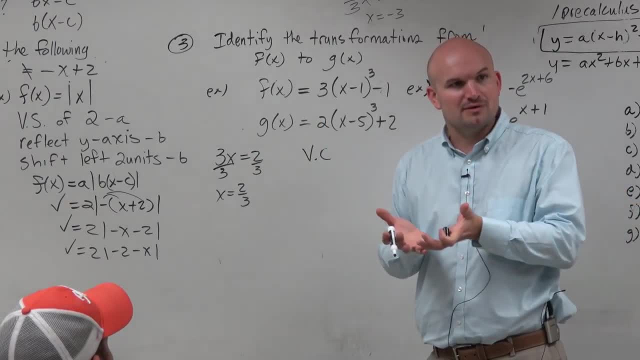 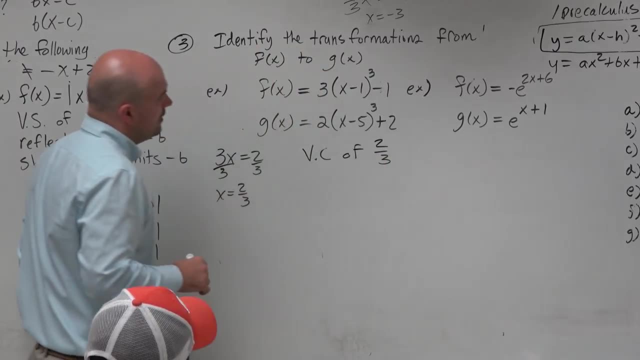 And people say, oh, fraction, it's a compression. Well, 3 halves, guys, is larger than 1, right, So just be careful with that. So it's a vertical compression of 2 thirds, All right for the next one. 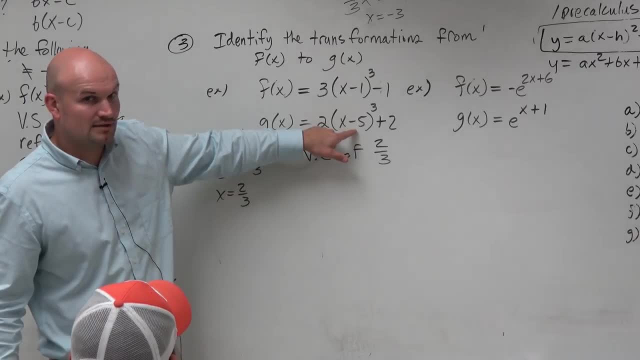 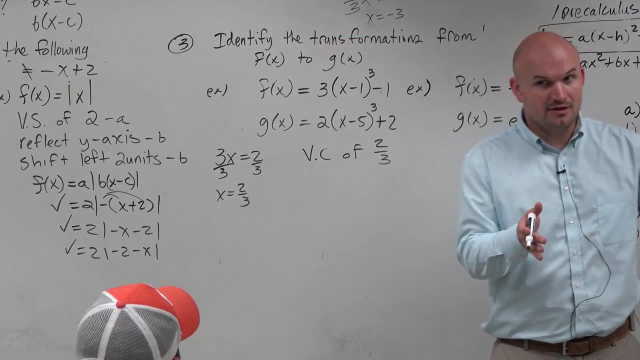 This one is left 1, and you need to go to left 4, or left 5.. So how do you do that? So here you are. One graph is left 1.. You need to get to left 5.. So what do you need to do? 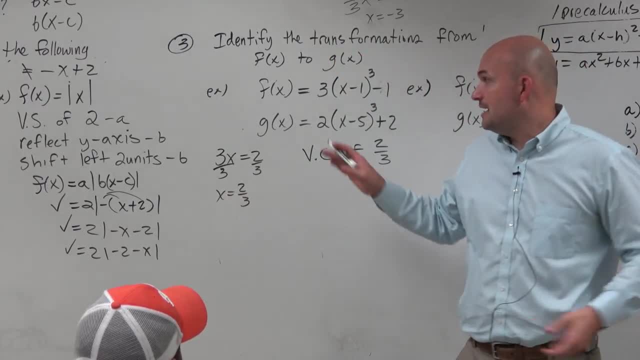 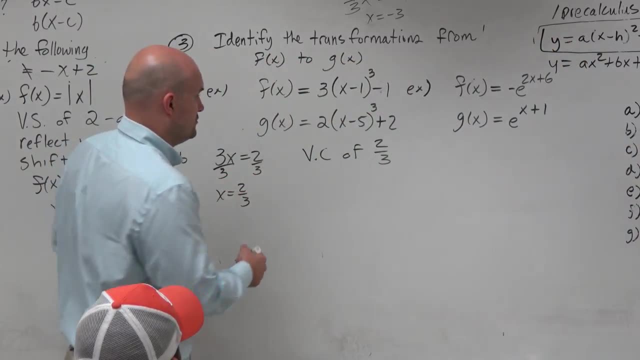 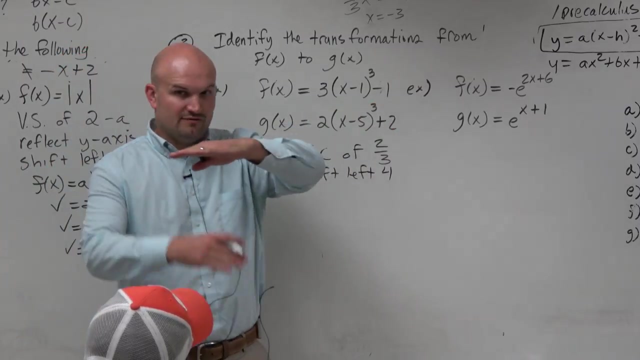 Well, you need to go left 4 more units right. And again, remember we're talking about addition and subtraction, so only talk about addition and subtraction. So, yeah, You need to shift left, 4.. And then, if I'm at negative 1 and I need to get up to positive 2,. 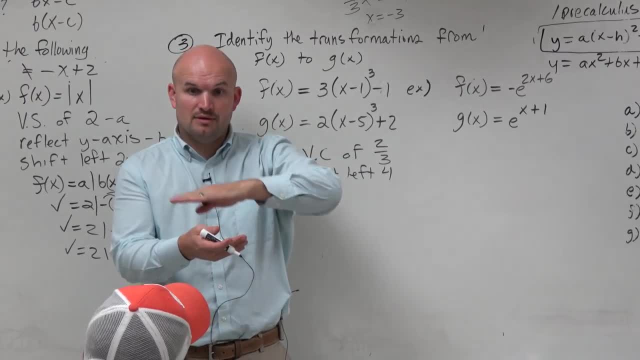 that means I need to go negative 1 up there. So you just say shift up 3..